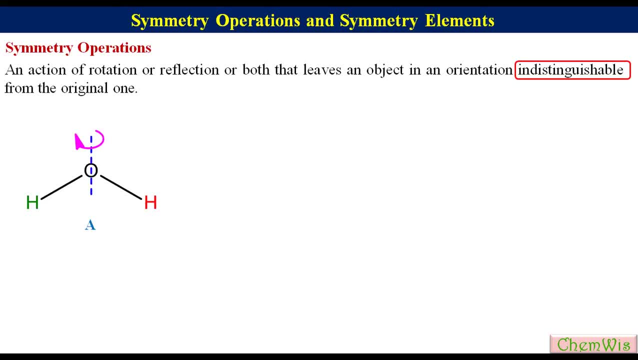 A through 180 degrees about this axis, we would get orientation B with green hydrogen on this side the right and red hydrogen on the left. Here we can see that original orientation A and orientation B obtained after 180 degrees rotation are different, or we can. 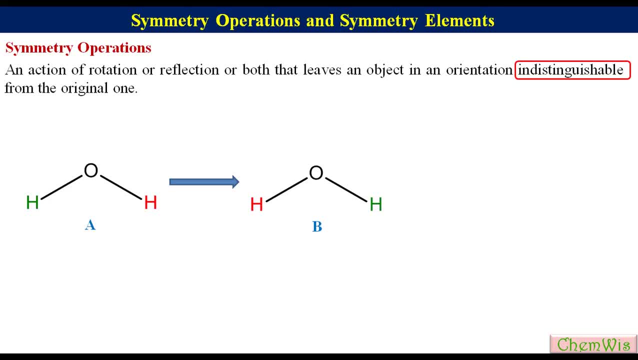 say distinguishable because we have colored the two hydrogen atoms But in reality both the hydrogen atoms are the same. If the two hydrogen atoms are of the same color, as in the case of real scenario, say black color, Under that condition we can say that the two hydrogen atoms are of the same color. 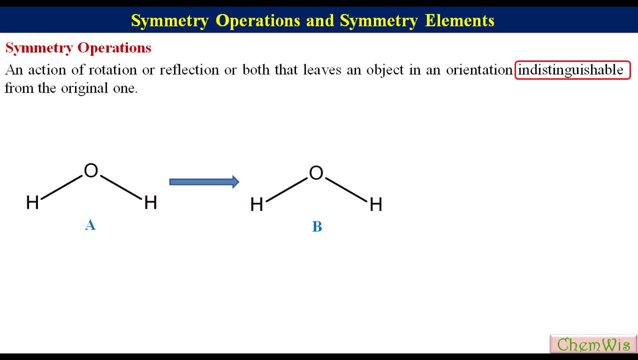 Under that condition we cannot distinguish between orientation A and B. Means orientation B obtained after rotating orientation A through 180 degrees is indistinguishable from the original orientation A. If we rotate B about this axis it will give orientation C. We can see that orientation C and original orientation A cannot be distinguished. 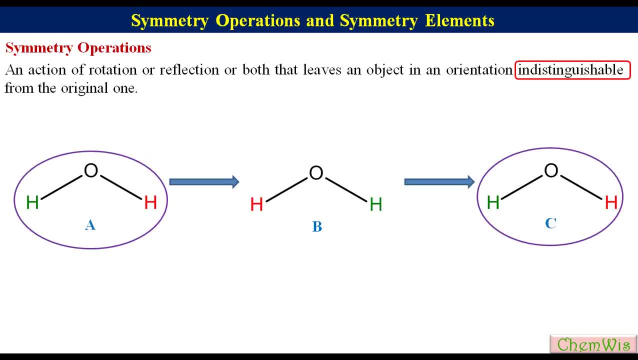 even if we have differently colored hydrogens. So orientation B is called equivalent orientation, while orientation C is called identical orientation. Symmetry elements. A symmetry element is a line, a plane or a point in or through an object about which a symmetry operation is performed. There are five types of symmetry. 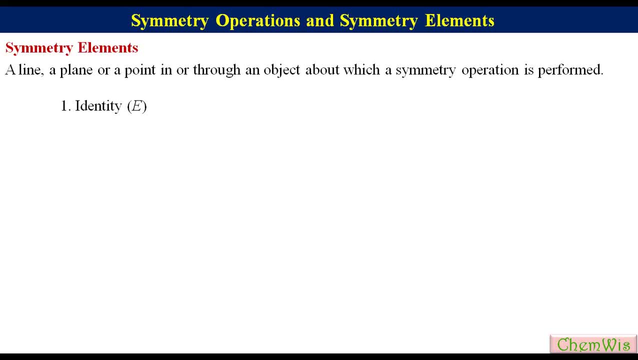 elements: 1. Identity, given by the symbol E. 2. Proper axis or rotational axis of symmetry, designated by Cn. 3. Plane of symmetry or mirror plane, designated by Sigma. 4. Center of symmetry or inversion center, given by I. 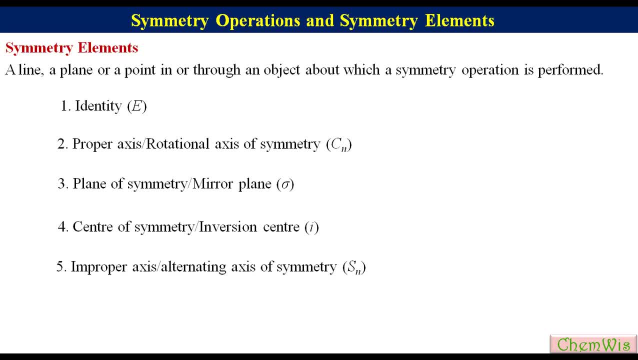 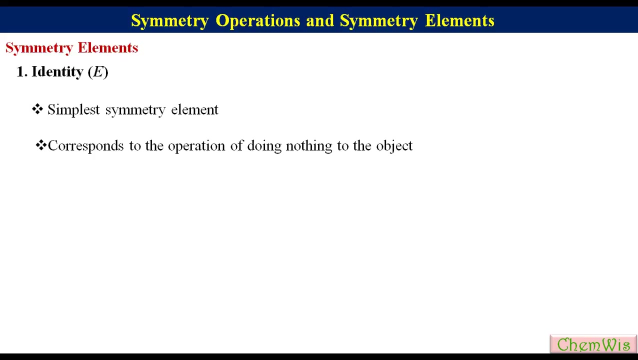 5. Improper axis or alternating axis of symmetry denoted by Sn. Now lets discuss one by one Identity. The identity symmetry element is the simplest symmetry element. It corresponds to an operation of doing nothing to the object. Every object possesses identity. 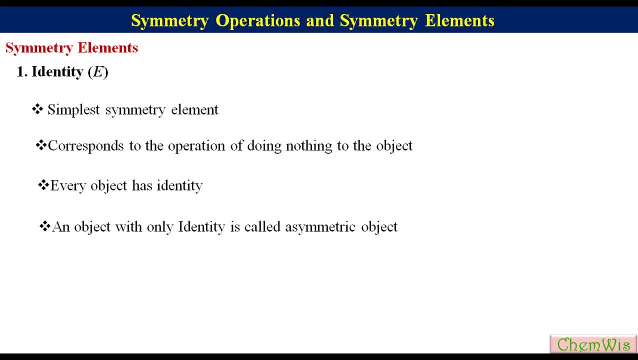 If an object possesses only identity symmetry element, the object is said to be asymmetric. For example, CHFCLBR. If we see its 3D structure we will find that it does not have any element of symmetry except identity. So this is an asymmetric object. 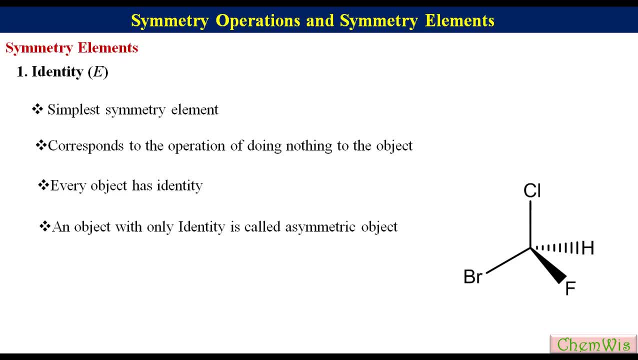 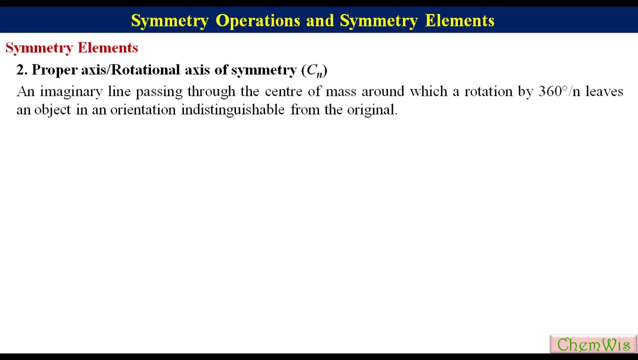 an asymmetric object is called a propagator. Proper axis of symmetry is an imaginary line passing through the center of mass, around which a rotation by 360 degrees upon n leaves an object in an orientation indistinguishable from the original one. situations of типography, vectorığı and. 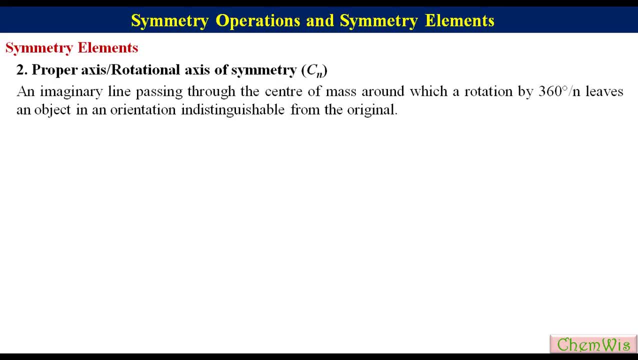 augmentation, since the contrivuration lasts much longer than integer內Annum and linear Zeit. a rotation by 360 degrees upon n leaves an object in an orientation indistinguishable from the original one. Theїn Crossway Line. ashm productorиж study". 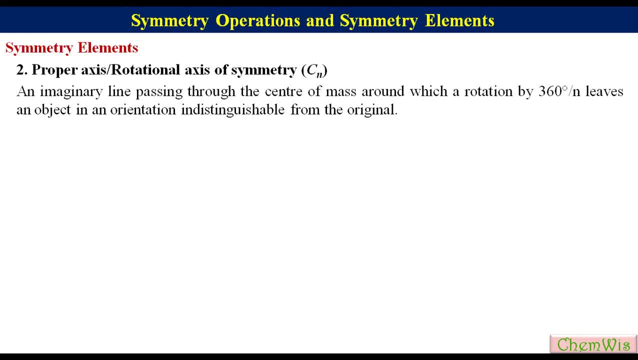 is called n-fold axis, abbreviated by cn, where n is an integer called order of axis. So an axis is called c2. if 360 degrees upon 2 is equal to 180 degrees, rotation around it leaves the object in an orientation indistinguishable from the original one. Similarly for c3 degree. 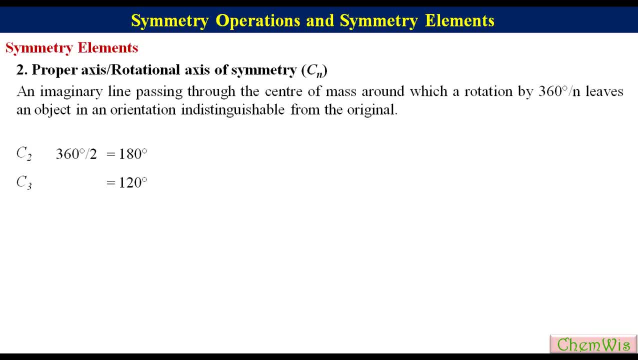 of rotation is 120 degrees, for c4 it is 90 degrees, for c5 it is 72 degrees, for c6 it is 60 degrees, etc. A c1 axis corresponds to a 360 degree rotation, and so it is the same as identity. 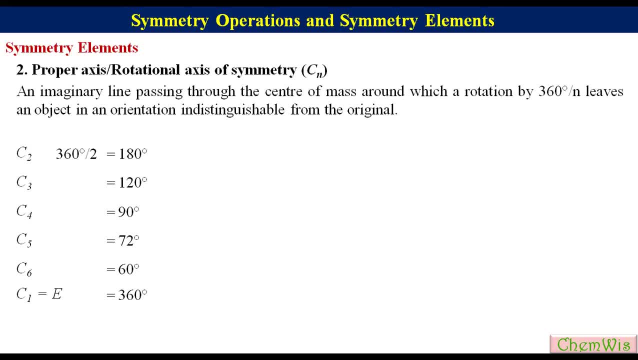 If a molecule possesses more than one type of cn axis, the axis of highest value of n is called the principal axis. If there are several cn axis of highest order, then the principal axis is the one passing through the maximum number of nuclei. We will discuss these two points with examples in details later. 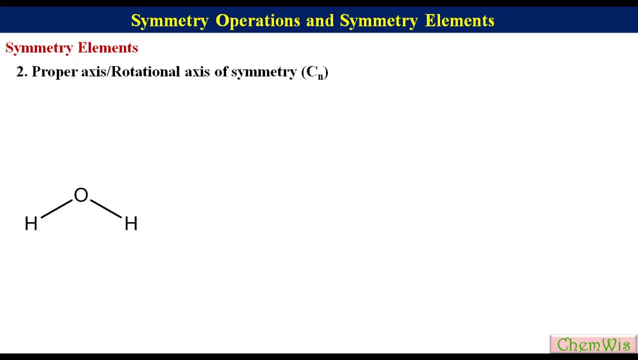 Lets take the example of water molecule For the better understanding. label the left hydrogen as 1. And the right one as 2.. Let this orientation denoted by a Draw, an axis passing through the center of mass. If we rotate water molecule around this axis through 180 degrees, it will give orientation. 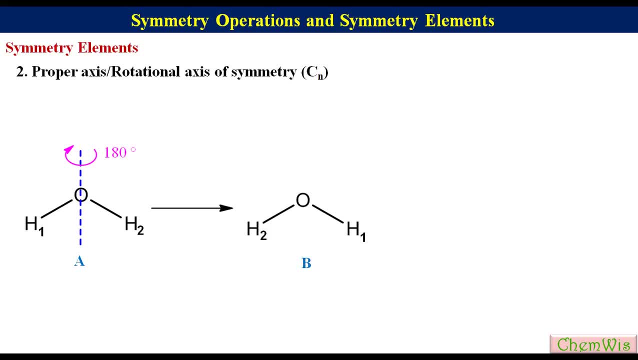 b, which is indistinguishable from the original orientation a. So, for the better understanding, label the left hydrogen as 1. And the right hydrogen as 2.. The order of the axis will be: 360 degrees upon 180 degrees is equal to 2.. 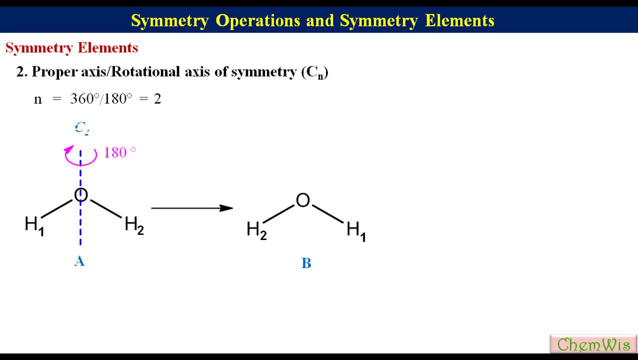 So we can say that water has c2 axis of symmetry. If we look at this structure, we will find that the respective positions of the hydrogen atoms have been changed. So we can say that the positions of hydrogen atoms have been changed. So we can say that the positions of hydrogen atoms have been changed. 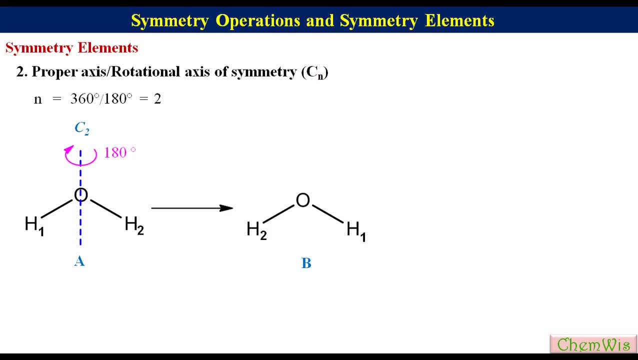 So this orientation is called equivalent orientation. If we rotate orientation b again about this axis through 180 degrees, It will give orientation c in which the respective positions of hydrogen atoms are same as original orientation a. So, for example, This is the original orientation a. 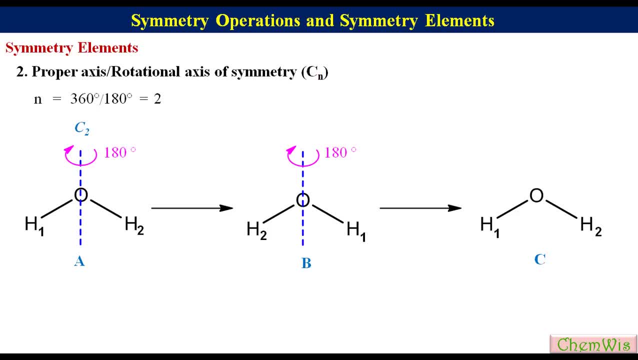 So If an inês nu- that means the original- lies with the current orientation A, the burst C is identical to A Since the two successive C2 operations led to the identity. so we can write: C2 square is equal to E. Ammonia: The structure of ammonia is pyramidal. There are 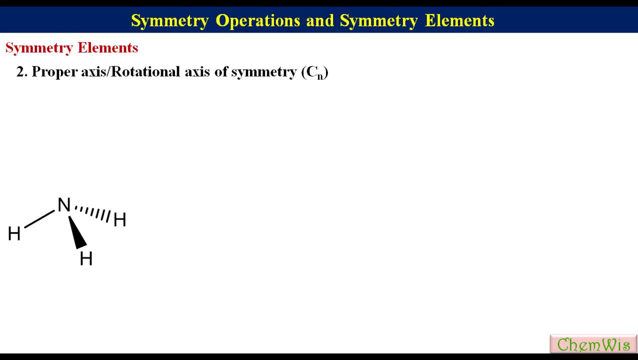 three equivalent hydrogens. Label them as 1,, 2 and 3.. Let this orientation be orientation A. Draw an axis passing through the center of mass. If we rotate ammonia molecule around this axis through 120 degrees, it will give orientation B. 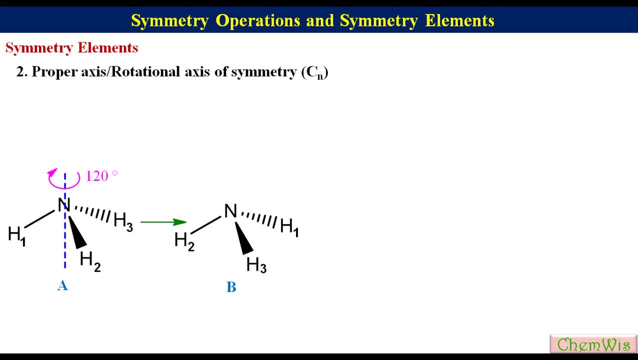 Which is Indistinguishable from the original orientation A. Order of the axis will be 360 degrees upon 120 degrees is equal to 3. So ammonia has C3 axis of symmetry. If we compare orientation A and B, we will find that the respective positions of hydrogen atoms have been changed. 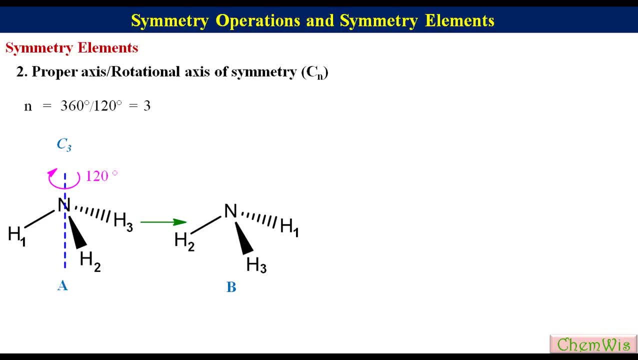 So this orientation B is called equivalent orientation. If we rotate orientation B again about this axis through 120 degrees, it will give orientation C, in which the respective positions of the hydrogen atoms are different from A and B. So C Is 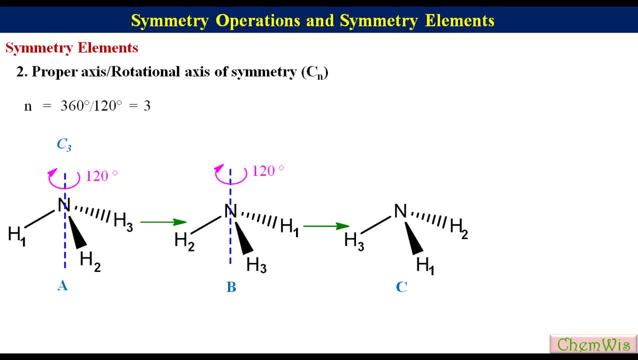 Also An Equivalent Structure to A. If we rotate orientation C again about this axis through 120 degrees, it will give orientation D in which the respective positions of the hydrogen atoms are the same as orientation A. So D Is. 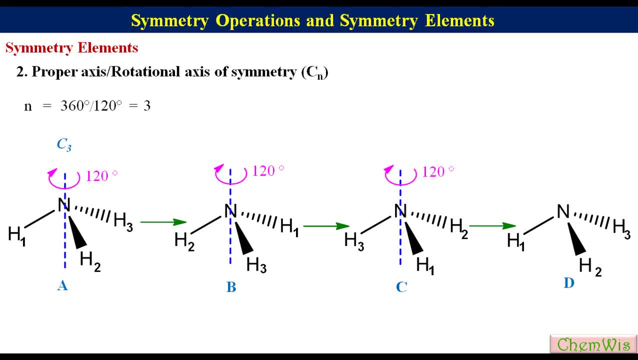 An Equivalent Orientation to A, Since the three successive C3 operations led to the identity, so we can write: C3 cube is equal to E. Boron trifluoride. The structure of boron trifluoride is planar, trigonal. 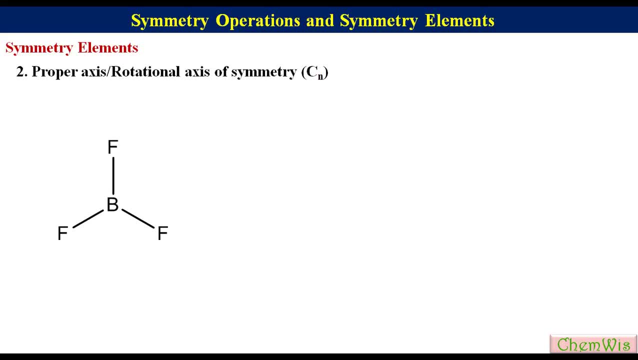 There are three types of boron trifluoride. There are three equivalent fluorine atoms. There are three belongs to the same host, which means the number of boron is different: E is equal to E and B is equivalent to C. 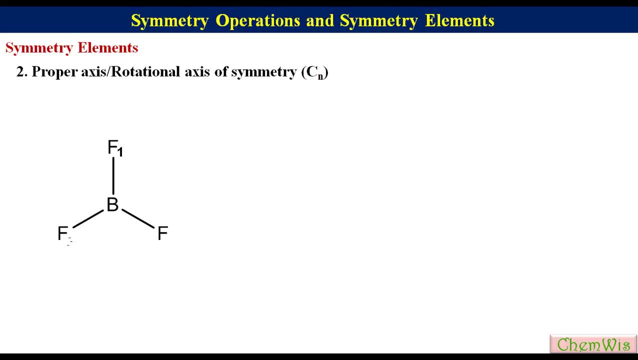 So for the two, we can label them as 1, 2 and 3.. There are three equivalent fluorine atoms. Label them as 1, 2 and 3.. The three have three c2 axes. We can see that there are three c2 axes present in the plane of the molecule and passing through 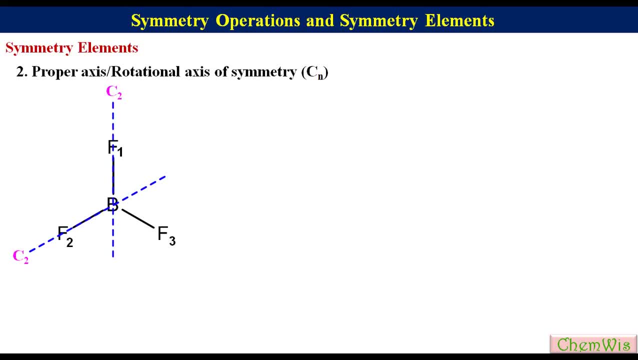 the BF1,, BF2 and BF3 bonds. If we draw BF3 molecule in such a way that the molecular plane is perpendicular to the plane of the paper, we can see that there is a C3 axis lying perpendicular to the plane of the molecule and passing through the boron atom. So there are four. 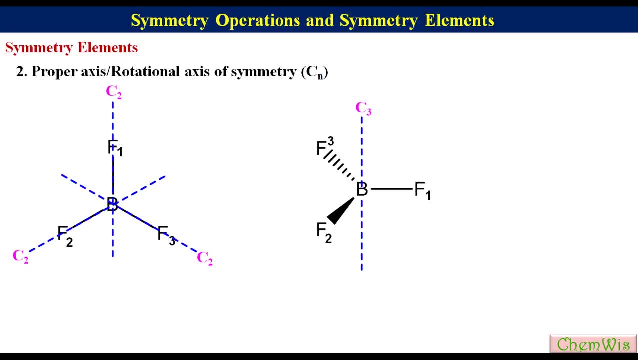 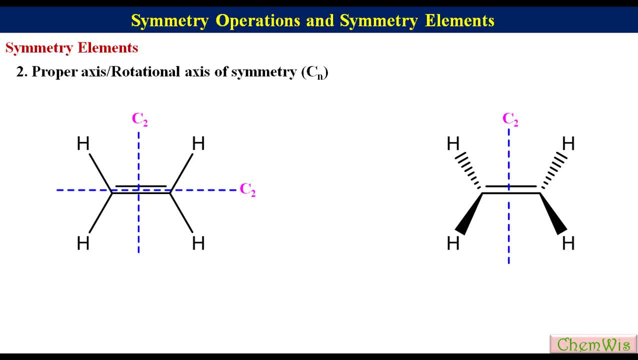 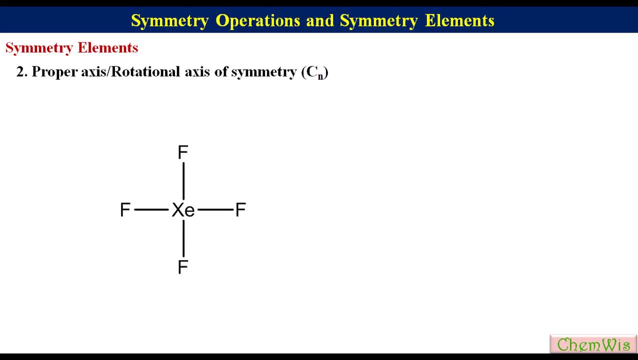 hydrogens Methane. The structure of methane is tetrahedral. There are four equivalent. hydrogens Methane. The structure of methane is tetrahedral. There are four equivalent needed—the rotor of basisine melody. Remember that如 in the sequence below 5. 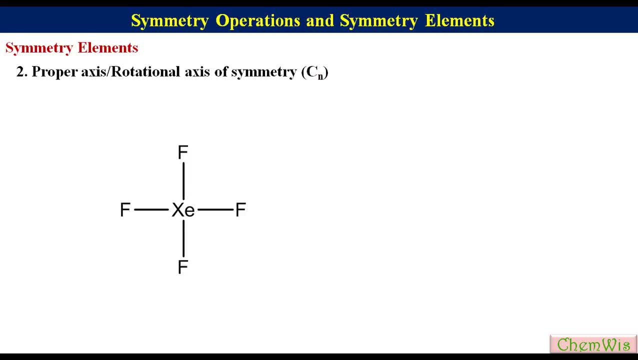 아� chegρ lässt raιsmețim σ". demonstrate compound clauses: 로 rams and rose water match. All the three axes have the same order. So in this case We will find that there are four C2 axes lying in the plane of the molecule. 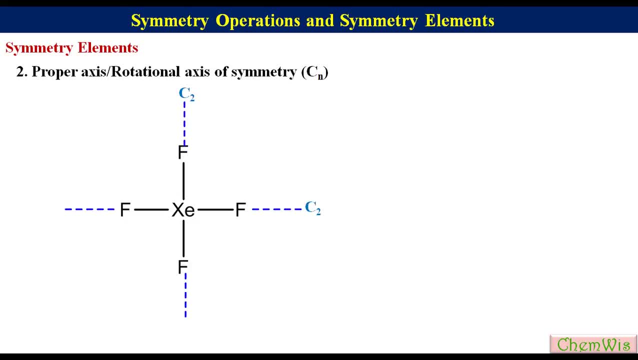 Two passing through the F-XCF bonds and remaining two bisects the adjacent bond angles. If we orient the molecule like this, we will find that rotation about this axis through 180 degrees or 90 degrees gives indistinguishable orientations. So this axis acts both as C2 and C4.. 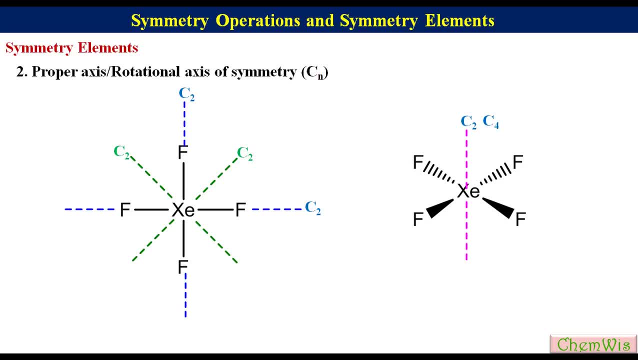 So in XCF4. There are five C2 and one C4 axes. C4 axes with the highest order will be the principal axes, The two C2 axes shown by the green color bisect, the bond angle and also bisect angle between. 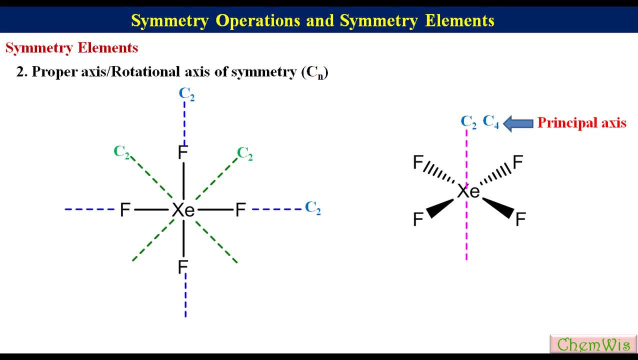 the two C2 axes. So these are called dihedral axes. Lets have XCF4 drawn like this: Label the four fluorine atoms as 1,, 2,, 3 and 4.. Label this orientation as A. If we rotate it about this axis through 90 degrees, we will. 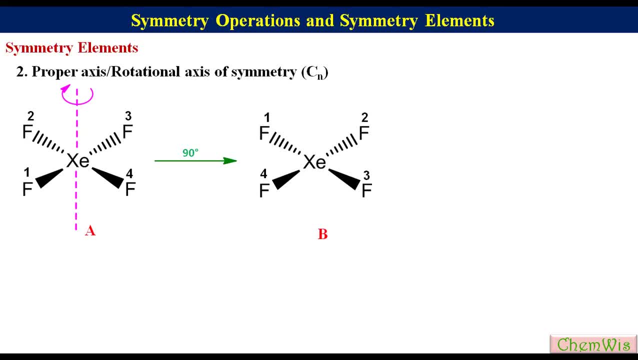 get orientation B. If we again rotate orientation B around this axis through 90 degrees, we will get orientation C. We can get orientation C directly from orientation A by rotating orientation A about this axis through 180 degrees. Thus We can say that two successive C4 operations, that is, C4 square, is equal to one C2 operation. 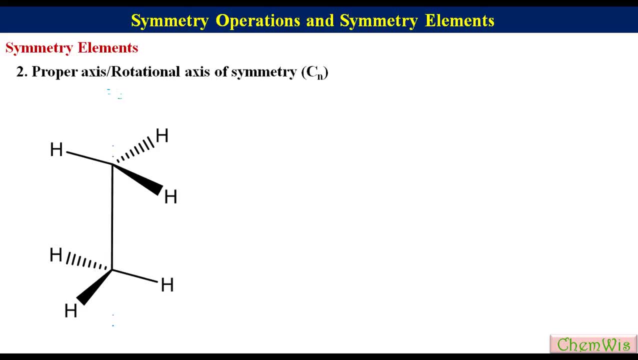 Staggered ethane. It has C3 axis passing through C-C bond. If we draw its Newman projection, We will find that There are one, two and three C2 axes perpendicular to C3, passing through the middle of C-C bond. 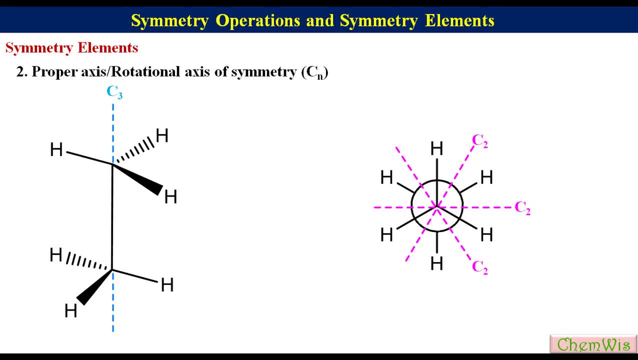 bisecting the dihedral angles. C3 axis is the principal axis because it has highest order. Eclipsed ethane, It has C3 axis passing through the C-C bond. C3 axis is the principal axis because it has the highest order. 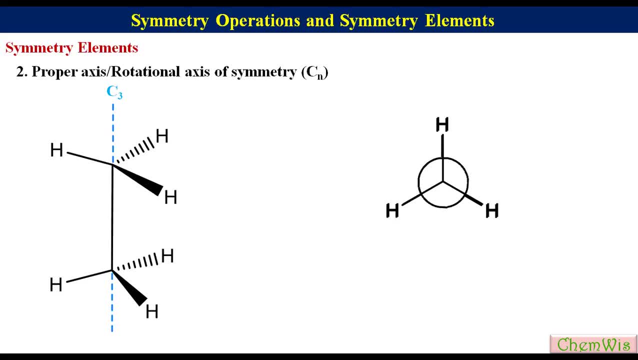 Eclipsed ethane. If we draw its Neumann projection, we will find that there are 1,, 2 and 3 C2 axes perpendicular to C3, passing through the middle of HCH bond angle. C3 is the principal axis because it has highest order. 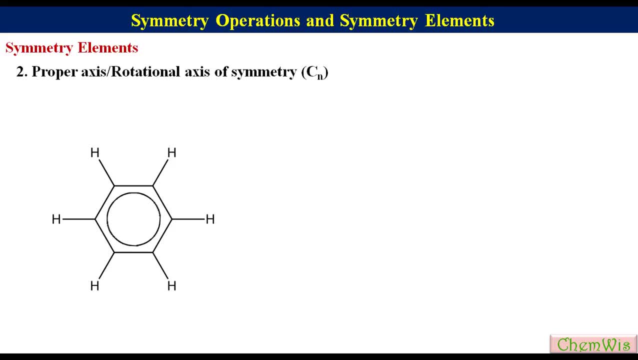 In benzene, there are 6 C2 axes present in the plane of the ring, out of which 3 pass through the carbons, making 1-4 relation, and 3 pass through the mid of the C-C bonds, making 1-4 relation. 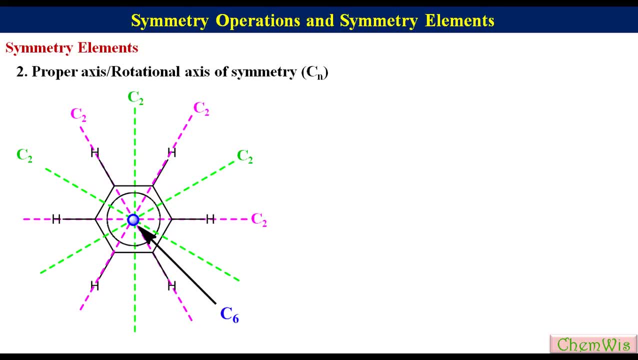 There is a C6 axis. It is perpendicular to the plane of the ring, passing through the center of the molecule. It will be more clear if we draw the benzene like this. This is the C6 axis. This axis also acts as C3 and C2 because rotation about this axis through 120 degrees and 120. 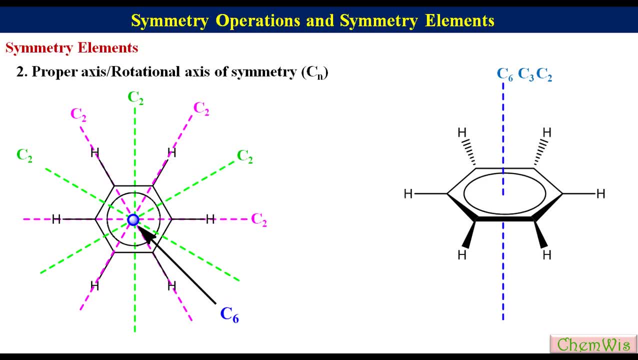 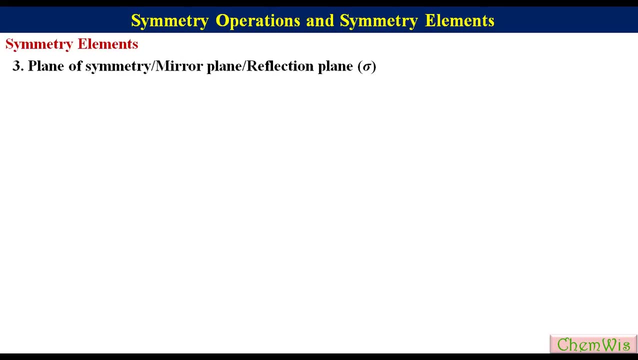 180 degrees give equivalent orientations. C6 axis is the principal axis because it has highest order. Now we will discuss plane of symmetry, mirror plane or reflection plane. A plane of symmetry or mirror plane or reflection plane is an imaginary plane which divides an object into two equal hubs which are mirror. 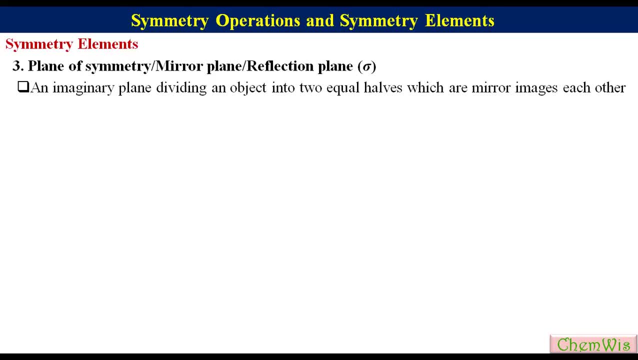 images of each other. In a reflection operation. two parts of an object after reflection through a plane produce an indistinguishable orientation. Each mirror plane has only one operation associated with it. Two successive reflection operations lead to identity, So we can write sigma square. 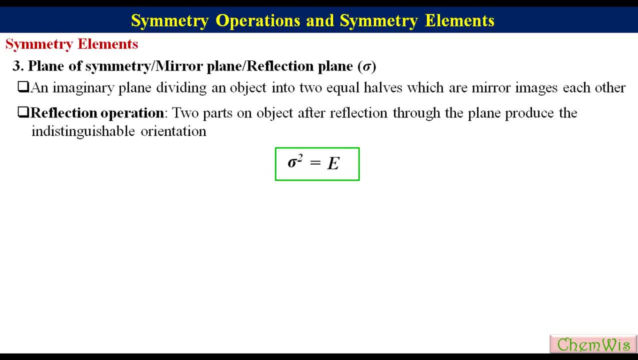 is equal to E. Mirror planes are of three types: Horizontal mirror plane, denoted by sigma h, vertical mirror plane, denoted by sigma v. and dihedral mirror plane, denoted by sigma d. Sigma h is perpendicular to the principal axis. Sigma v contains principal axis passing through the maximum number of atoms and. 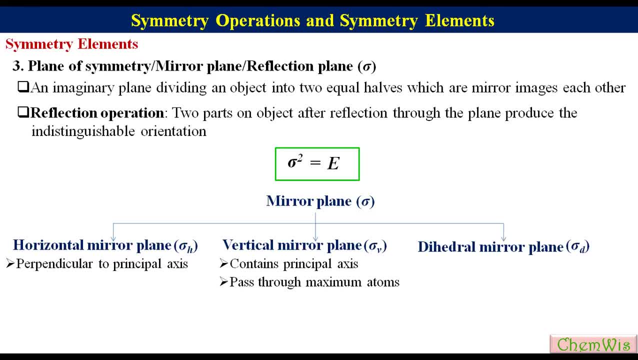 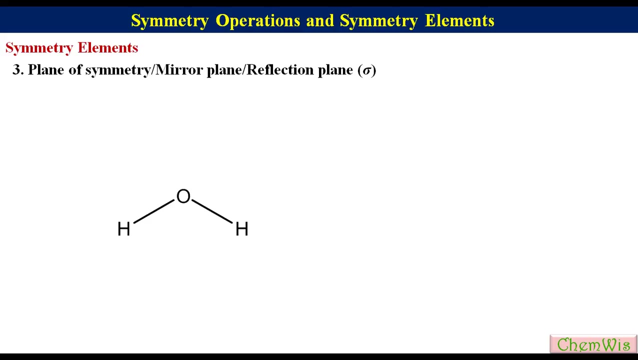 sigma d also contains principal axis, but it passed through the less number of atoms. It is an angle bisector between two C2 axes. It typically bisects bond angles. Let us take the example of water molecule. As we have already discussed, this is the C2. 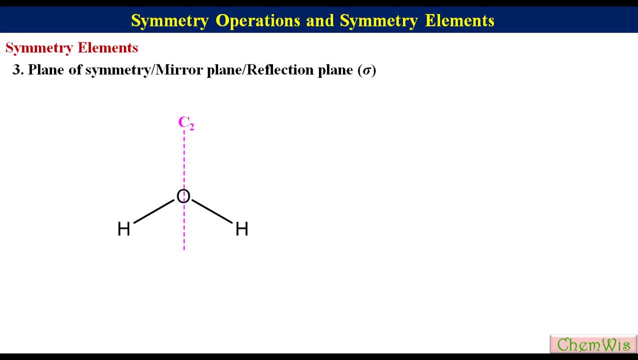 and principal axis. There is a plane containing this axis That divides every atom into two equal hubs. This plane is shown by sigma v. There is one more plane containing principal axis that bisects the HOH bond angle, and this plane is designated as sigma v prime. 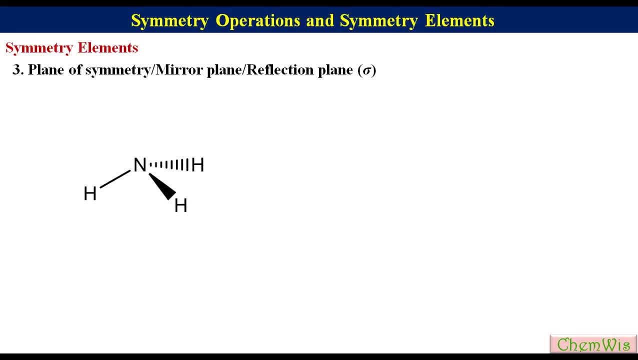 Ammonia. In the case of ammonia, there is a C3 axis that acts as principal axis. For the better understanding, let us have top view of this molecule. If we bisect this molecule by an imaginary plane like this, we will get two equal hubs. 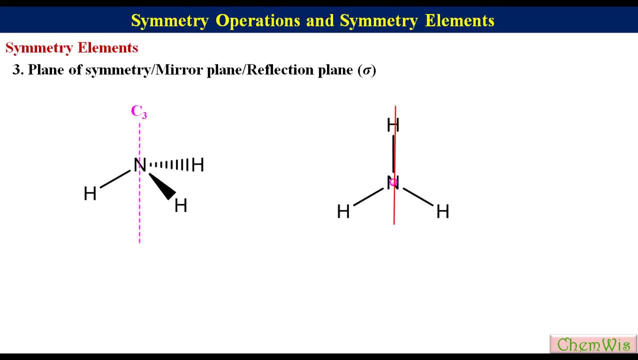 which are mirrored images of each other. Since this plane contains principal axis, so it is a sigma v. Similarly, there are two more sigma v's, So there are three vertical plane of symmetrical in ammonia molecule Xcf4.. We have already discussed that there are four C2 axes in ammonia, from four C1 to C2 axes. 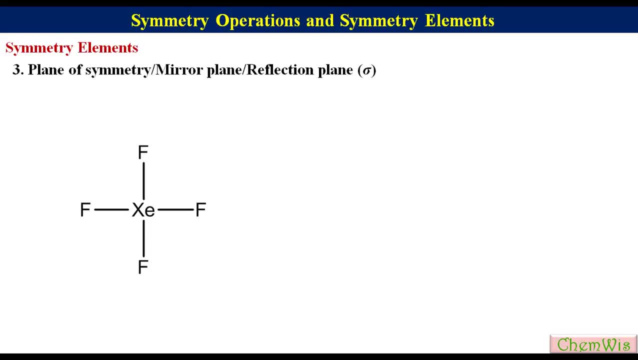 of the molecule out of which to pass through the f-axi-f bonds and the remaining to bisect the adjacent f-axi-f bond angles. There is a C4 axis perpendicular to the plane of the molecule. This axis also acts as C2 axis. 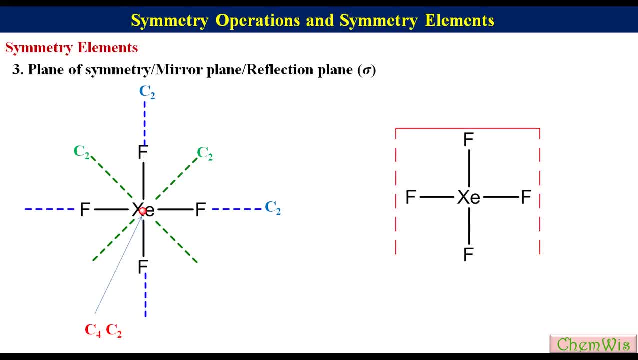 The plane perpendicular to the principal C4 axis bisecting each atom is designated as Sigma H. There are four vertical Sigma planes containing principal axis and bisecting two C2 axis, out of which two bisect, two fluorine and one xenon atom. 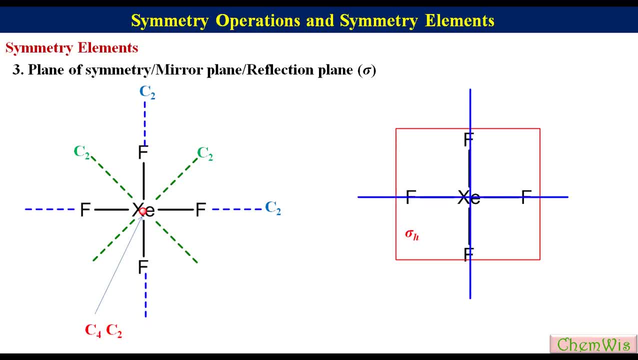 While remaining two bisect only xenon atom. The blue planes containing the greater number of atoms are designated as Sigma V, while pink planes containing less number of atom, that is, only xenon atom. bisecting angle between two C2 axis and also two bond angles are designated. 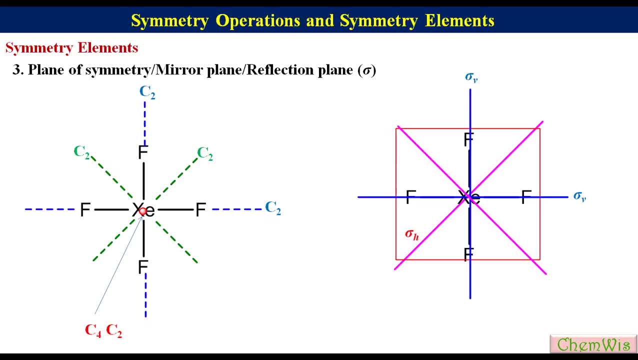 as Sigma V Alene. It contains a C2 axis along the molecular axis. There are two more C2 axis perpendicular to the principal axis, passing through the central carbon inclined at 45 degrees to the CH2 planes at either end of the molecule. 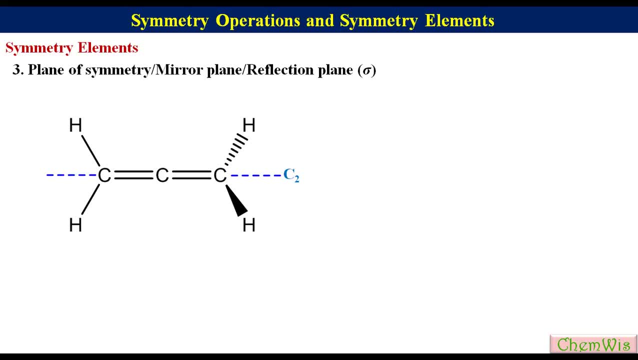 For better understanding of the C2 axis. please refer to the video on the left hand side of the screen For better understanding of these two axes. let's make Neumann projection of Alene. These are the two axes we were talking about. There are two mirror planes. since both are 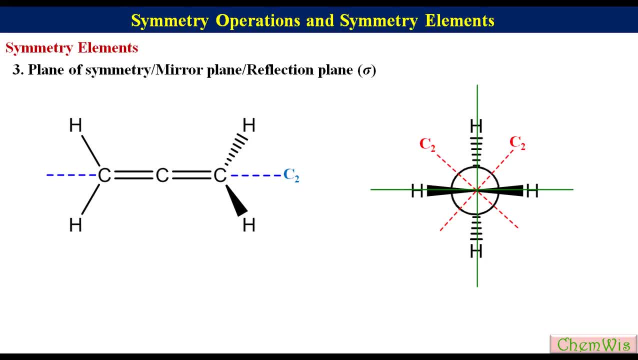 along the principal axis and bisect angle between two C2 axis, as well as bond angle. So these are designated as Sigma D 2,2-dichloro-alene. In this principal axis is C2.. There are two vertical planes perpendicular. 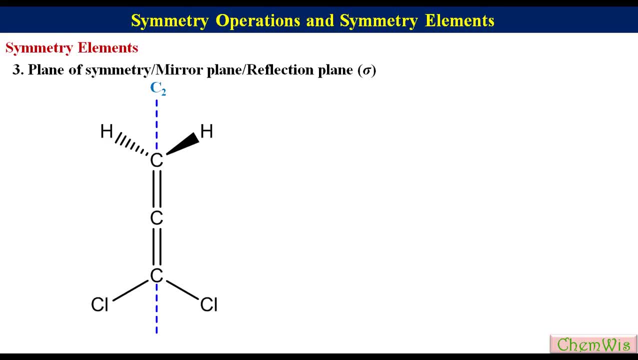 to each other. Out of two planes, one bisects H-C-H bond angle, while other bisects C-L-C-C-L bond angle. These are designated as Sigma V Staggered ethane. As we have already discussed, it has a C3 axis passing through the central. 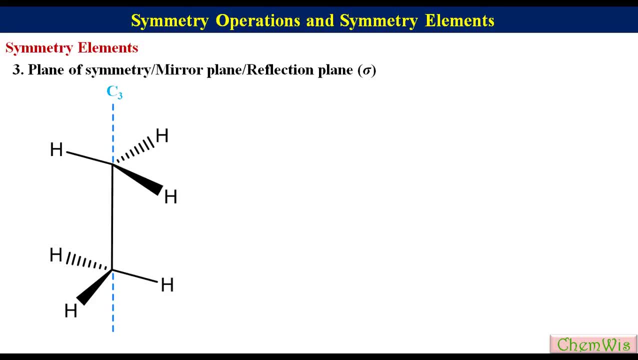 axis passing through the C-C bond and three C2 axis perpendicular to the C3, passing through the middle of C-C bond, bisecting the dihedral angles. There are three vertical planes bisecting the bond angle, as well as the angle between: 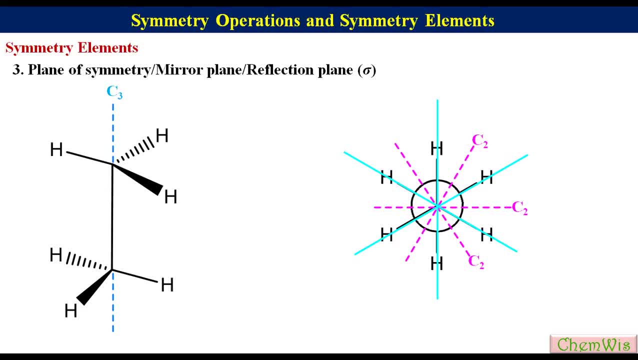 two C2 axes, So These are designated as Sigma D- Chair form of cyclohexane. In chair form of cyclohexane, three alternate carbons go upward, while remaining three go downward. Let the carbons going upward denoted by blue spheres. 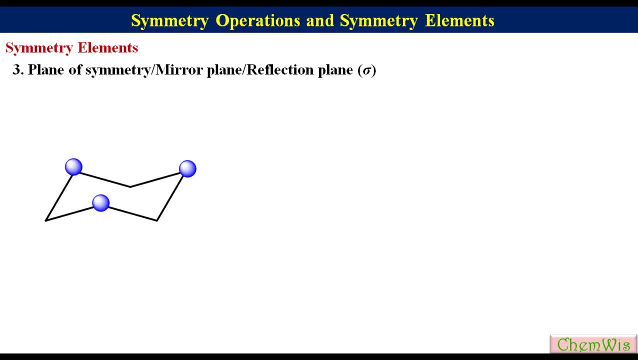 while those going downwards by red spheres, We can see that there is a C3 axis There. It would be more clear if we draw the top view of the molecule. Here the center represents C3 axis. There are three C2 axes perpendicular to the C3 axis, bisecting C-C bond making 1-4 relation. 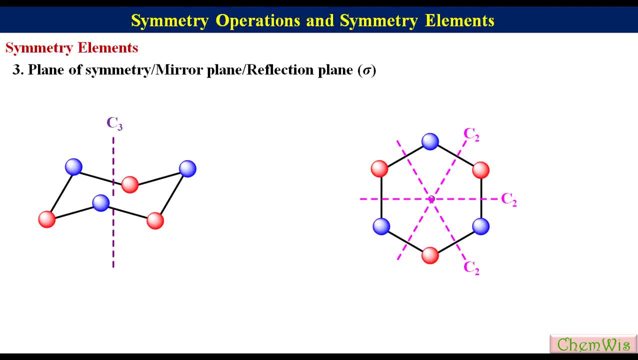 There are three mirror planes that bisect two C-C-C bond angles, making 1-4 relation, and also bisect bond angle between two adjacent C2 axes. So these are designated as sigma d. Now come to the fourth point: center of symmetry or inversion center. 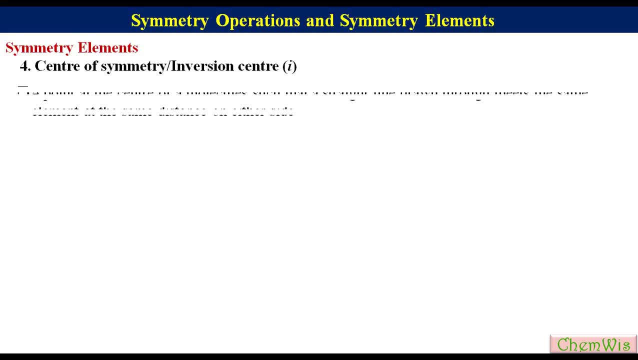 Inversion center. Inversion center is a point at the center of a molecule, such that a straight line drawn through it meets the same element at the same distance on either side of the molecule. In inversion operation, every atom or group of a molecule is reflected through the inversion. 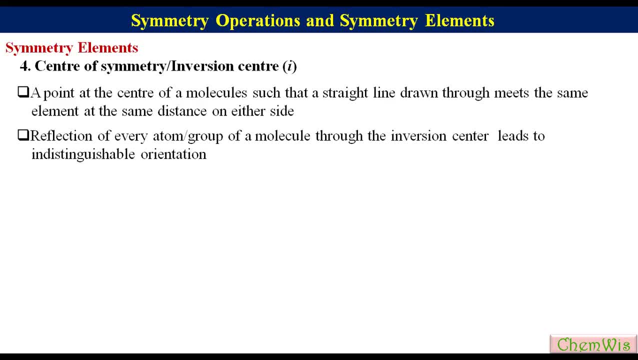 center that results indistinguishable orientation: Plainer, trigonal, pyramidal, tetrahedral, trigonal bipyramidal square, pyramidal, pentagonal planar, pentagonal pyramidal and pentagonal bipyramidal structures don't have center of. 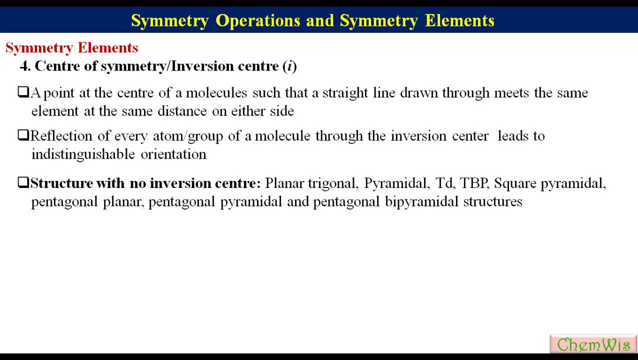 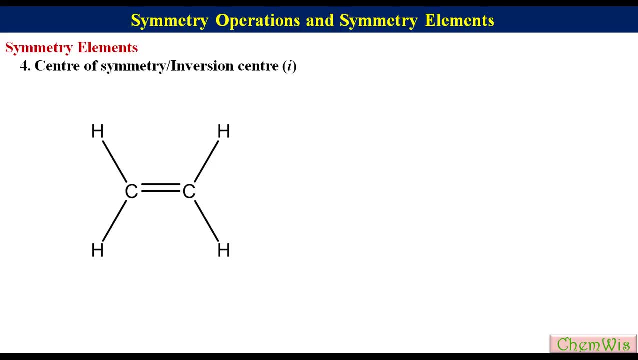 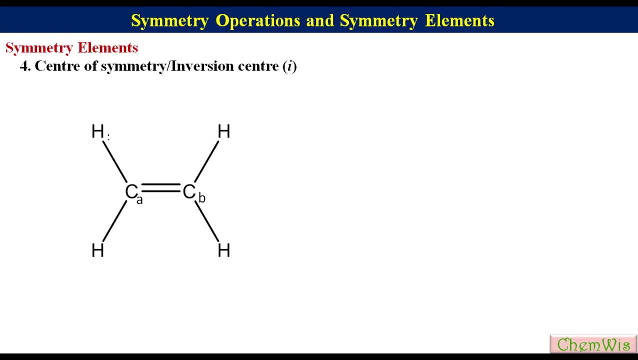 hydrogens as 1, 2, 3 & 4.. This is the center of molecule. If we draw a line between h1 and h3, it will pass through the center. The distance between the center and h1 will be equal to the distance between the center and h3.. 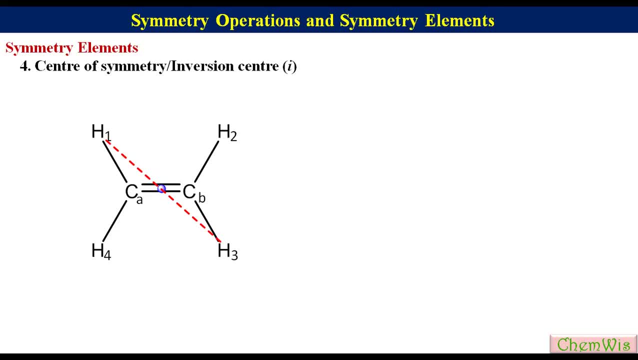 Okay, If we draw a line between h2 and h4, it will pass through the center meeting h2 and h4 at equal distance from the center. Similarly, a line drawn between C A and C B will pass through the center meeting C A and C B at equal distance from the. 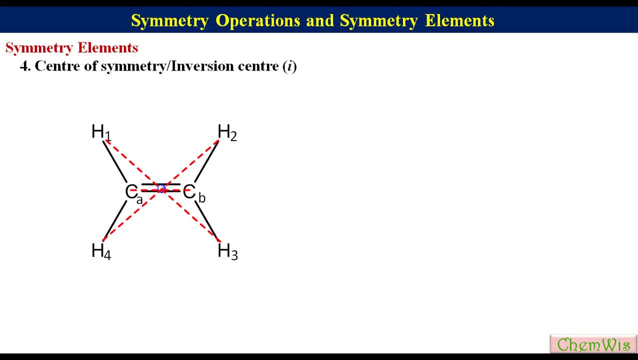 center. So So ethylene has center of symmetry. We can also find the center of symmetry by reflection operation. If we reflect all the atoms H1,, H3,, H2, H4 and Ca Cb through this center, it will give. 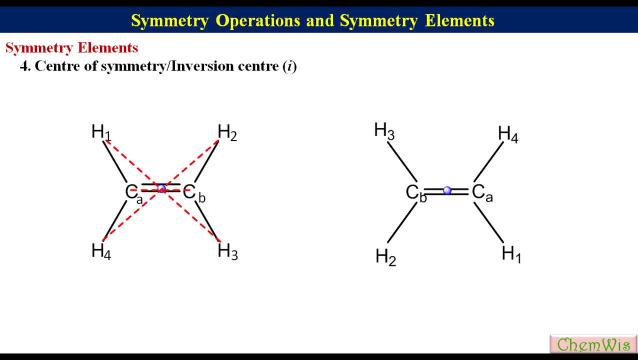 an orientation which is indistinguishable from the original one, PtCl4.. Let's first level the form 4 chlorine atoms as 1,, 2,, 3 and 4.. This is the center of the molecule where platinum is situated. 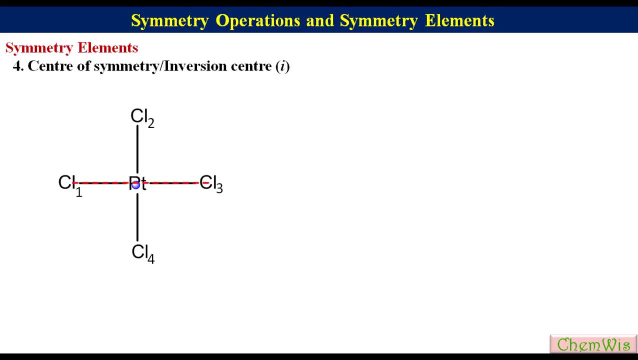 If we draw a line between Cl1 and Cl3,, it will pass through the center. The distance between Cl1 and center will be equal to the distance between Cl2 and the center. Similarly, if we draw a line between Cl2 and Cl4,, it will pass through the center. 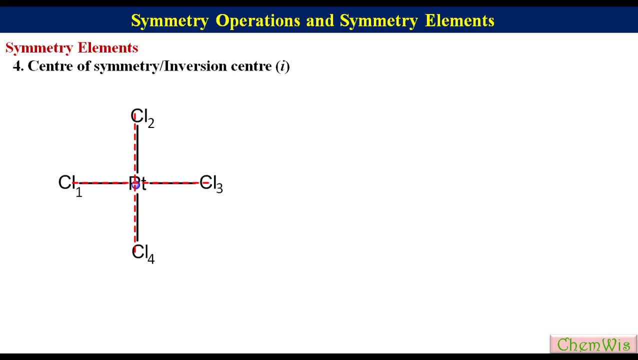 meeting Cl2 and Cl4 at the equal distance from the center. So PtCl4 has center of symmetry. We can also find the center of symmetry by reflection operation. reflection operation If we reflect the four chlorine atoms Cl1, Cl3 and Cl2, Cl4 through. 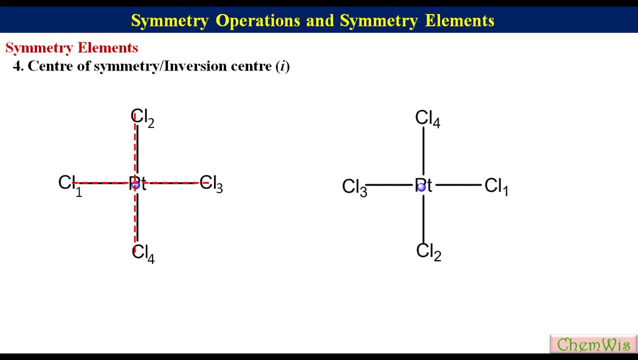 this center, we can see that the new orientation is indistinguishable from the original one. These are few more examples of molecules having center of symmetry: Carbon dioxide, trans-1,2-dichloroethene, trans-1,2-difluorodiazine, staggered ethane. 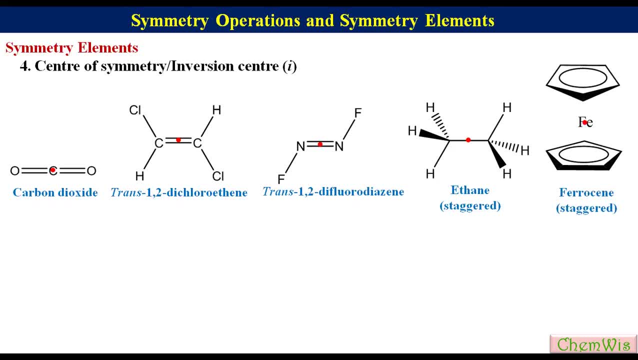 staggered: ferrocene, mesotartaric acid, benzene, cyclohexane, carbon dioxide, carbon dioxide, sulfur, hexafluoride, etc. Now come to the last point: Improper axis or alternating axis of symmetry An object. 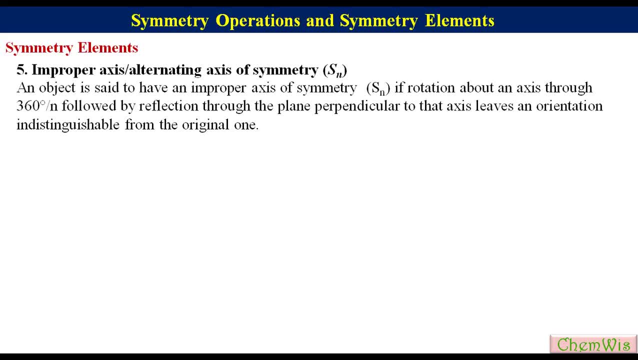 is said to have an improper axis of symmetry if rotation about this axis through 360 degrees upon n, followed by reflection through the plane perpendicular to that axis. So we can write Sn is equal to Cn into sigma h where n is greater than 2, because S1 is equivalent. 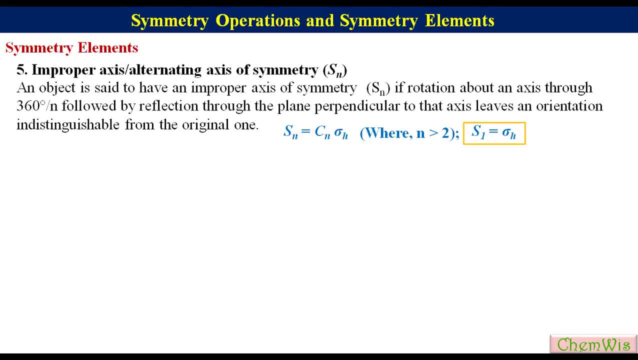 to sigma h and S2 is equivalent to i. The equation shows that if both Cn and sigma h exist, then Sn must exist. One more thing which one should remember is that neither Cn nor sigma h necessarily needed to exist for the existence of Sn axis. 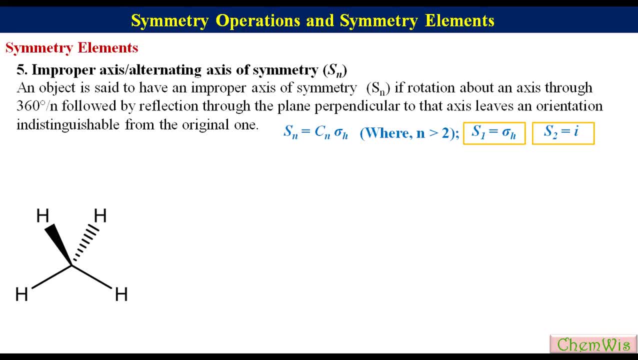 Lets take the example of methane. There are four equivalent hydrogen atoms. For the better understanding, label them as 1,, 2,, 3, and 4.. Let this orientation be labeled as orientation A. Rotation of this orientation about this axis through 90 degrees will give orientation B, which is the same orientation as orientation. a Rotation of rotation A is equal toburn to 1,, 3,, 1,, 2,, 3,, 4.. Rotation of rotation B is equal toburn to 1,, 3,, 1,, 2,, 3,, 4.. Rotation of rotation B is equal toburn to 1,, 3,, 2,, 3, and. 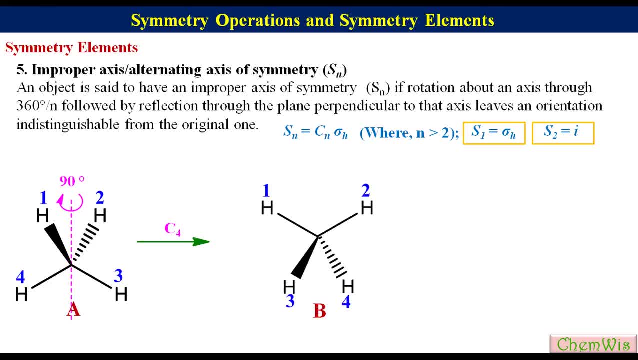 different. that is distinguishable from orientation A. Reflection of atoms through this plane perpendicular to the axis will give orientation C, which is indistinguishable from the original orientation A. So methane molecule has S4 axis of symmetry. There are total 3 s4 axis of symmetry in methane molecule. 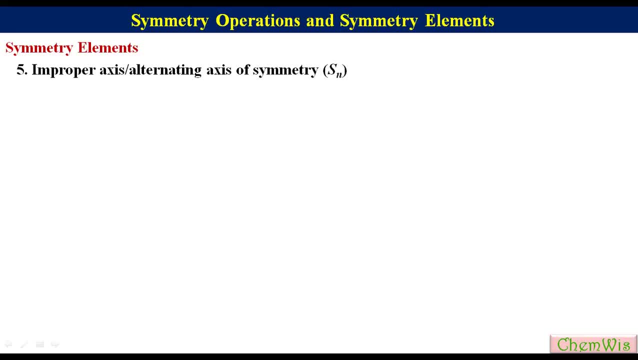 Similarly, in the case of eleene, rotation of orientation A about this axis through 90 degrees will give orientation B. This orientation is different that is distinguishable from the original orientation A. a reflection of atoms through this plane perpendicular to the axis will give orientation. 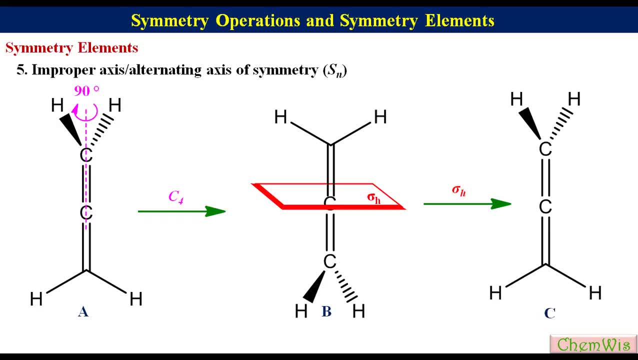 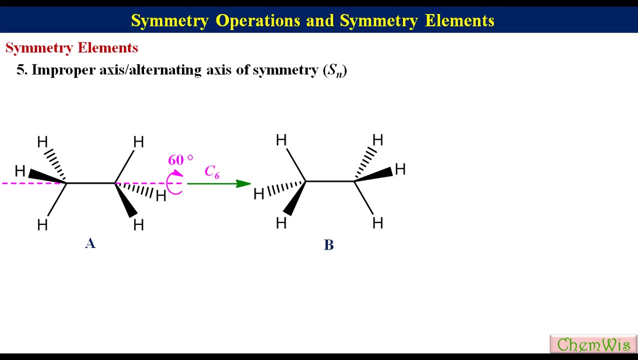 c which is indistinguishable from the original orientation a. so alien has s4. improper axis of symmetry, staggered ethane. let's label this orientation as a rotation of orientation a about this axis through 60 degrees will give orientation B, which is distinguishable from 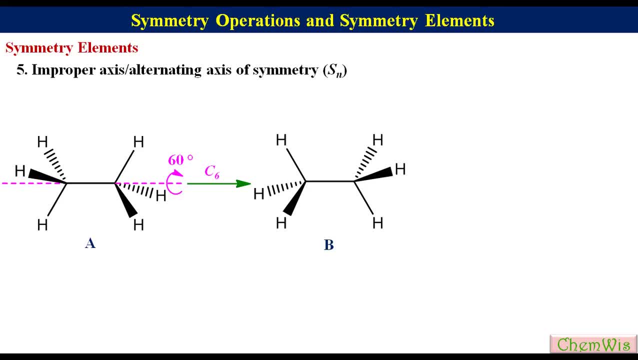 the original orientation a. reflection of atoms through this plane perpendicular to the axis will give orientation c, which is indistinguishable from the original orientation a. so staggered, ethane has s6 improper axis of symmetry. eclipsed ethane. for the sake of better understanding, protons have. 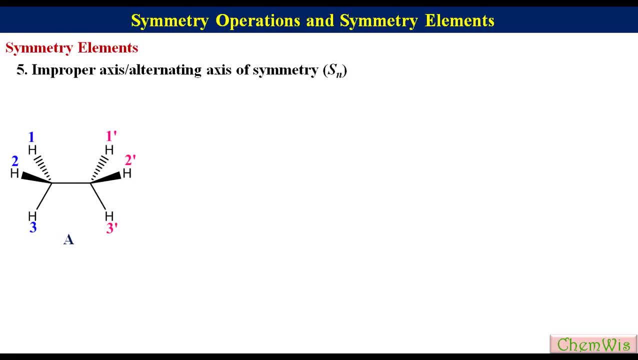 been labeled as one, two, three and two, and one prime, two, prime and three. prime. rotation of orientation a about this axis through 120 degrees will give orientation B, which is indistinguishable from the original orientation a. reflection of atoms through this plane perpendicular to the axis will give orientation c.